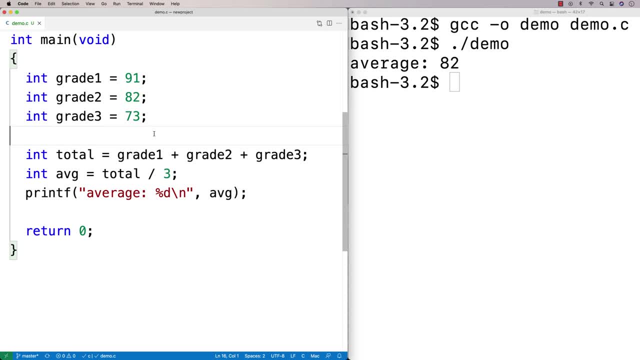 and now we have five students in our class. I could add two more variables here. but then anywhere in my program where I'm kind of using this group of variables together, I'd have to add the variables there too. And what if? in a more realistic kind of scenario, 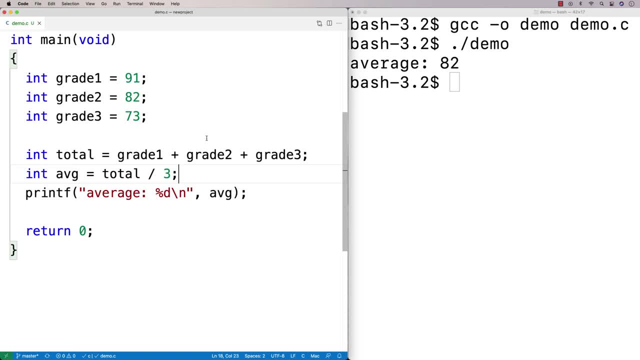 I don't have just have three students or five students in my class. What if I have a hundred? what if I have 1100 or 2000 in my class, which which happens in very large classes in you know, maybe, the first year of a college or something like that? what am I going to do? 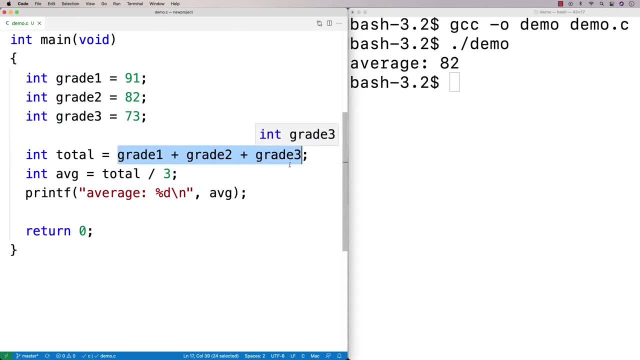 Am I going to have like 2000 grade variables that are all you know being added together like this? That's going to be a very large chunk of source code there, So this approach is not going to scale very well. We need a better way of representing a group of related data. 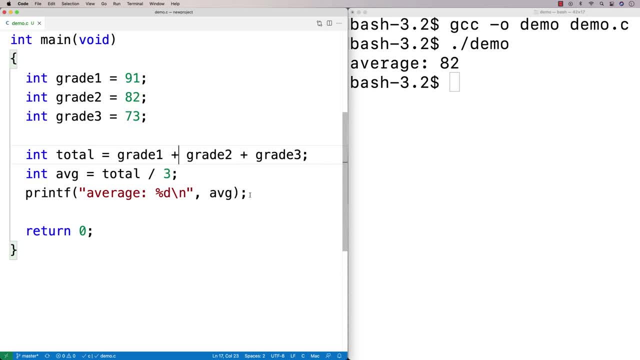 So let's do that with an array. So an array allows us to declare this collection of data That's going to have the same type and we're going to use the same name to address that data. So it looks like this: I'm going to say here, int grade, and I'm going to say 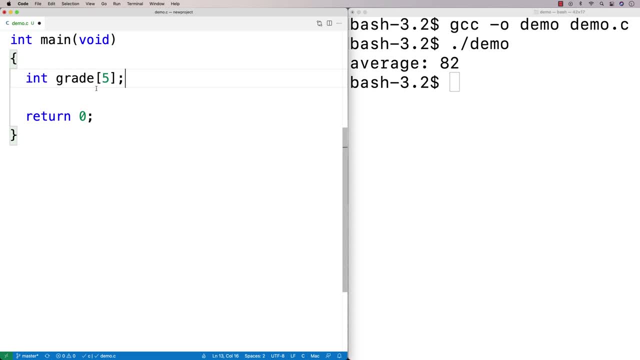 here five. So I'm going to say here int grade, and I'm going to say here five. So what this does is it declares a variable, that is an array called grade, and int means that grade is going to store integers And this open bracket. 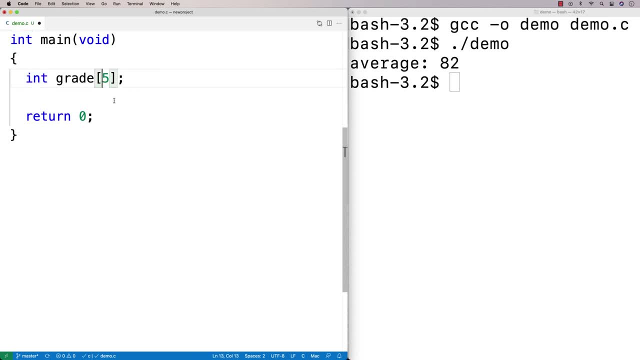 close bracket with the five in the middle there. that's saying that it's going to store five ints, So there's going to be space for five integers in this array here. So what we have in memory is something that looks like this: We have this grade array in memory. 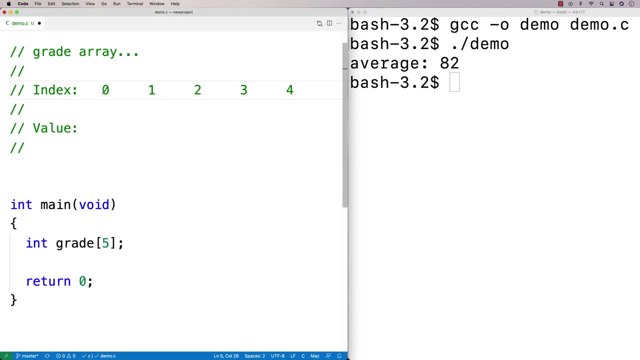 and we have basically five positions in memory And we access those positions in memory with what's called the index. So we have this index into the array and it actually starts from zero, which is kind of interesting. There's a lot of things in programming where you'll find that we 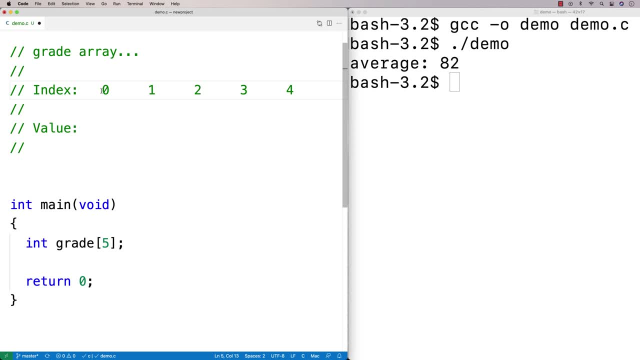 actually start counting from zero, and it's kind of a meme or a joke that programmers count from zero. But the first position in the array where we can store one of these five values is given by index value. Now, what? the way? what I could do is get a value these two different ways. 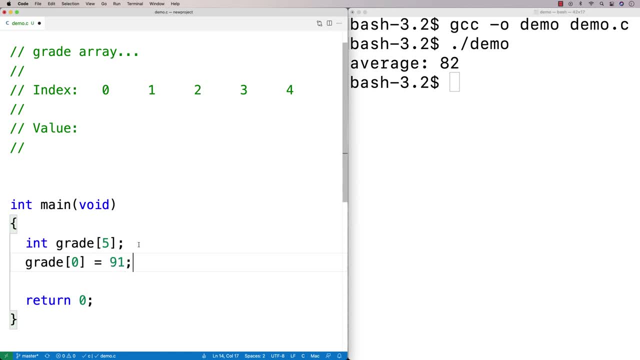 and all in random 층 or compound according to giving a value. So what I could do is I could say here, grade at zero is equal to, and I could say 91. And when I do that, what happens is, at this index zero in the grade array that stores five ends, we're going to store the value 91.. 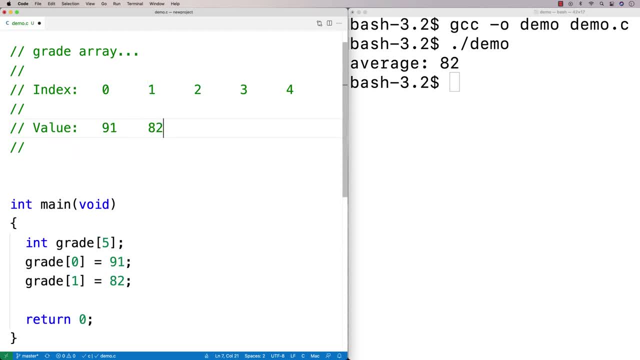 Graph, in case 0: 0.. and I can access these indexes as well and I can use them to do things like print. so I could say here like print f, and I could say grade. I'll say zero here is equal to percent d, and then I can. 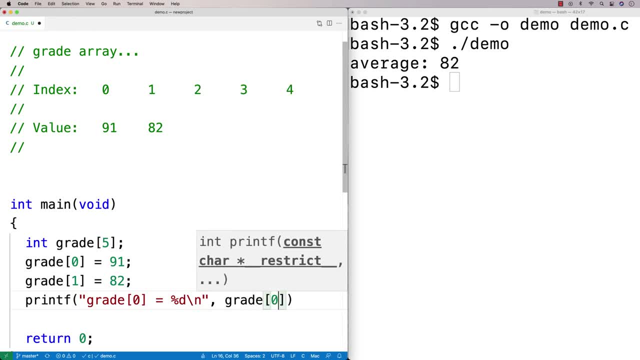 print out what grade at zero is, so I can use this grade at the zeroth index here like I can any variable. so if I save this here and run this, we'll be able to output that grade at zero is ninety one. and I could keep going here. so I could say, like grade at two is equal to 73, and again. 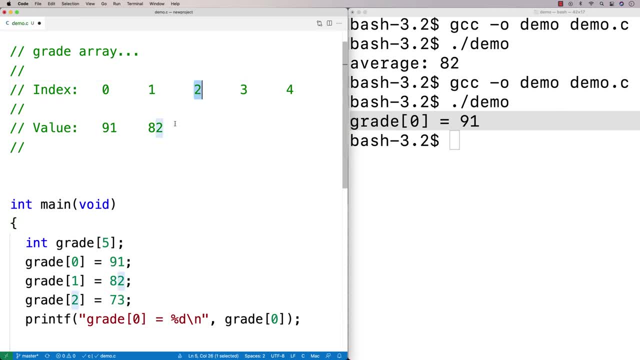 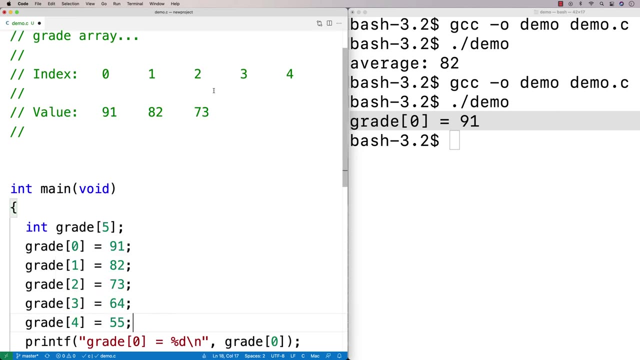 that's gonna basically fill in this index to position in memory in the grade array. that's, with 73 I could say grade three is equal to, and I'm gonna say here 64, and I'll say grade four is equal to two and I'll say 55. And then our array is going to look like this: I'm going to have 64 here at. 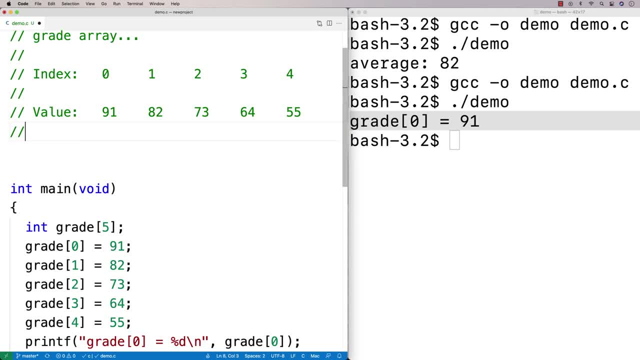 three and 55 here at four, And now I've got this group of data that I can work with and I can access the individual values in that array using the index. So each of these, like five values that we're storing. they're stored using an index and they start from zero and they go up until one less. 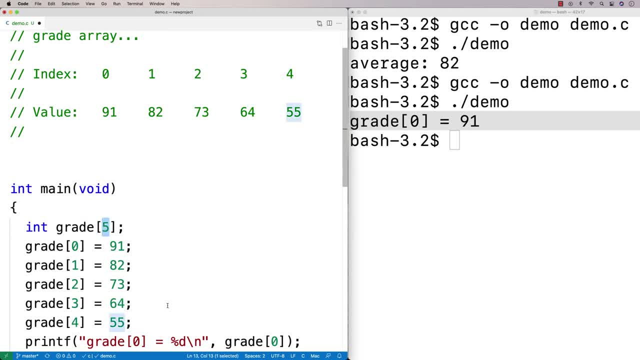 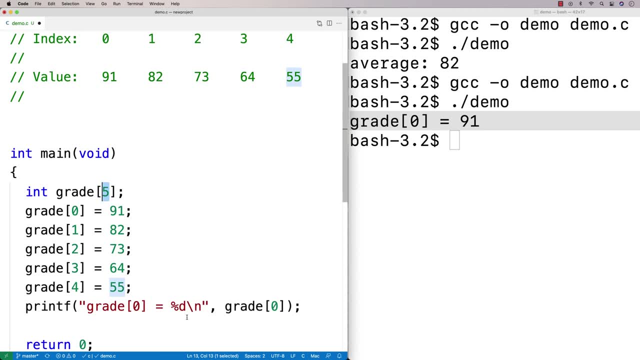 than the actual size of the array, because we start at zero And once I've got my data like this, I can actually make it easier to work with than if I had individual variables. So let's say I want to print out all the values in this array here. What I could do is I could have a series of print. 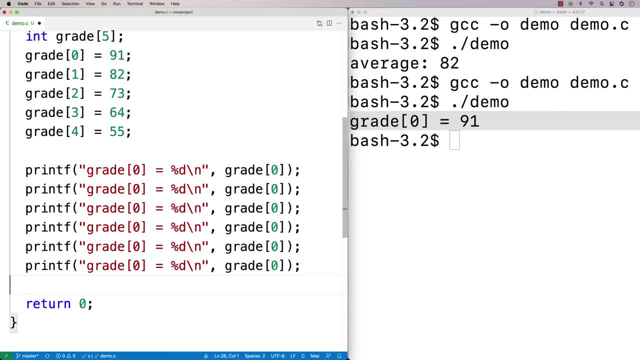 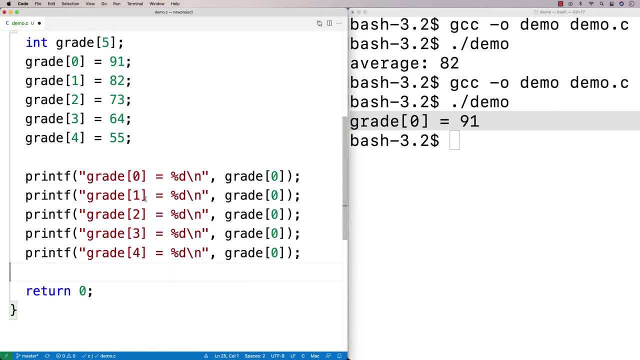 Fs. So I could say like print F, grade zero, and I'll make print Fs for the others as well. So we'll do like one, two, three, four and we don't really need this last one here. but we got one, we got. 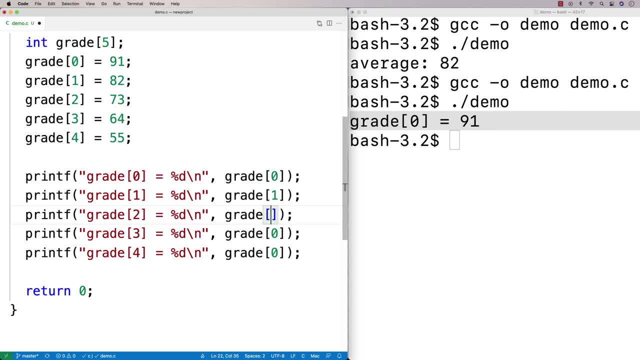 zero: one, two, three, four here, And I'm going to print Fs for the others as well. So we'll do like one, two, three, four and we don't print out grade at zero- one, two, three, four here- And this will print out all the grades, And so we could. 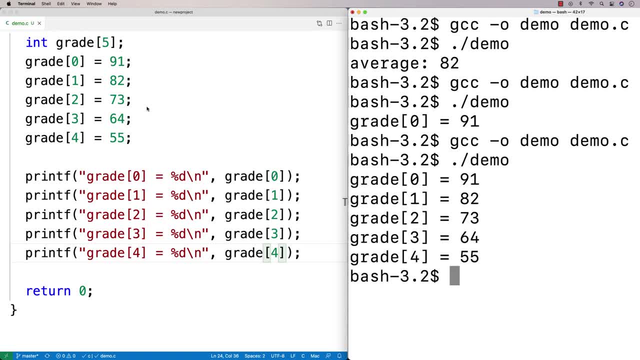 compile this and run it, And now we're printing out all the grades in our array here, And this is one way of working with this data. But now what I can do? because I can address the grades here in the array using this index, I can use a variable to access the data here. So let's say, for example, I do this, I say int, i is. 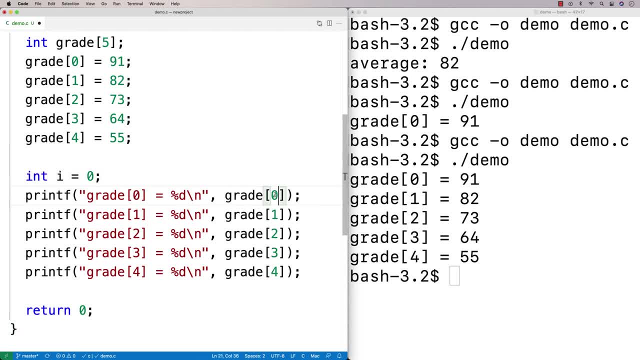 equal to zero. What I'm going to do is I'm going to print out the grade here according to i. So I'm going to say i. Now I'm going to say here, i plus plus, And I'll say i, i plus plus, And I'll say i, And I'll keep doing. 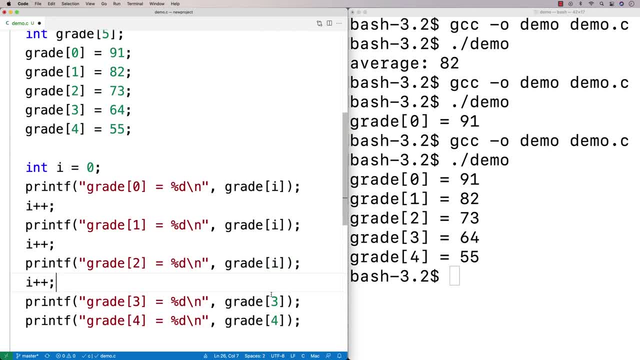 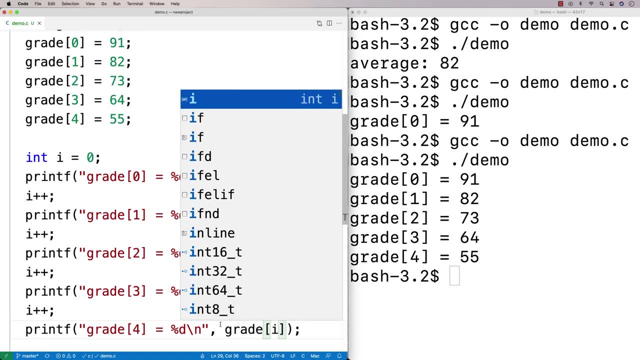 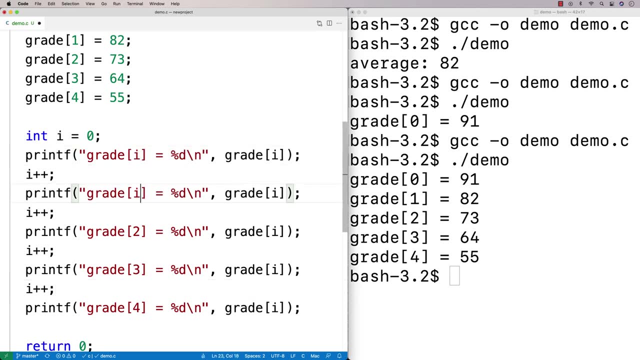 this: i plus plus, And then I'll say i, i plus plus, And then I'll say i. And what I'm doing here is I'm using a variable now to access the grades. So this is initially going to be percent d, And I could actually add an i here too. I might as well add it in here as well, Say, i say percent d. 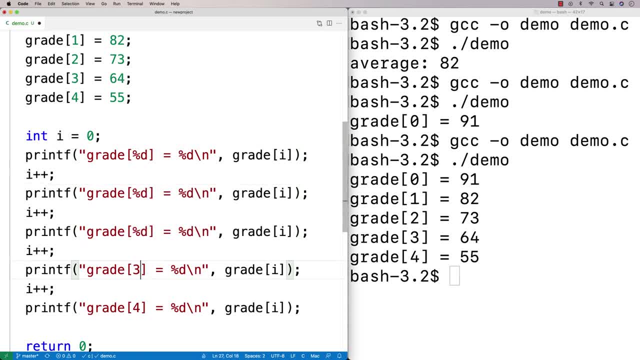 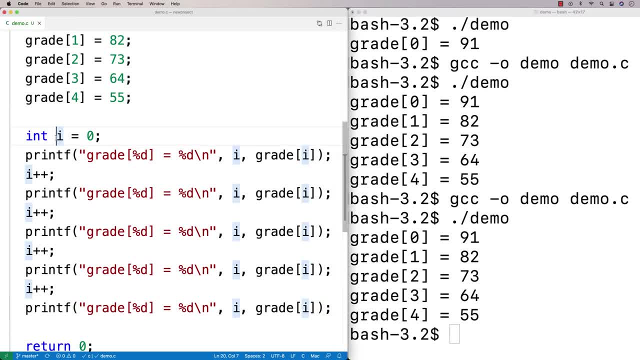 But the difference is now is I'm using this variable i to access the grade array And I'm modifying i, I'm incrementing it by one each time, So that way I'm accessing the next thing in the grade array with each subsequent printf. So what this allows us to do is write loops, And we can. 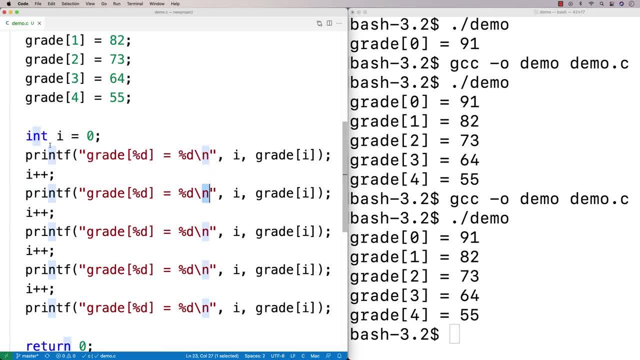 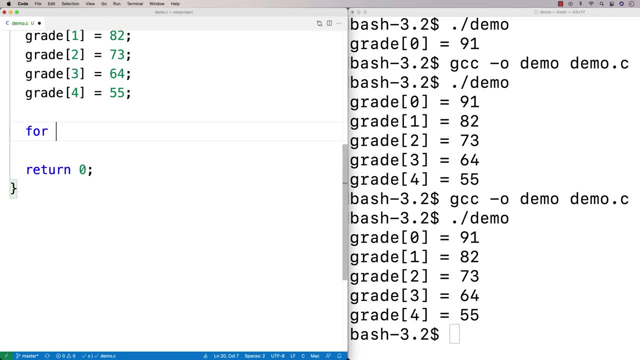 write loops that will actually work with our data now in an array according to some index variable that's probably going to be the counter variable for our array. So I could take this code and I could write it like this. I could say here: 4. And I'll say here: 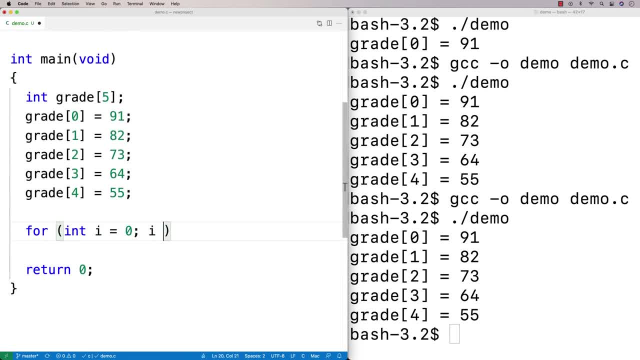 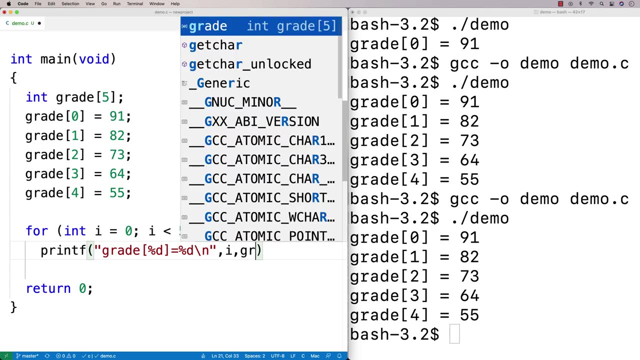 I'll say 4.. And I'll say int i is equal to 0.. i is less than 5.. i plus plus, And I'm going to say printf And I'll say grade percent d is equal to percent d. And then I'll say here: slash n i and. 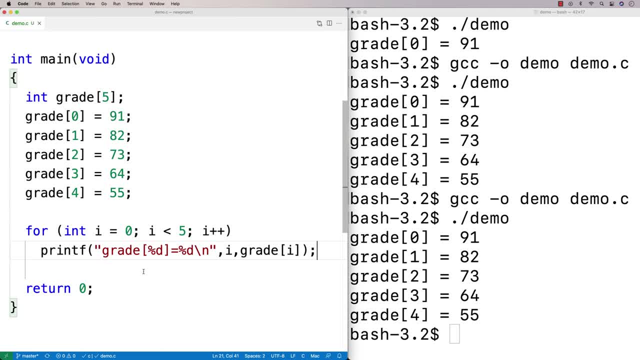 grade at i, And what I'm doing here is I'm printing out grade at i that starts at 0, there is equal to grade at i, which is the actual value in the array, And then I'm incrementing i by one each time. So I'm basically doing exactly what I had. 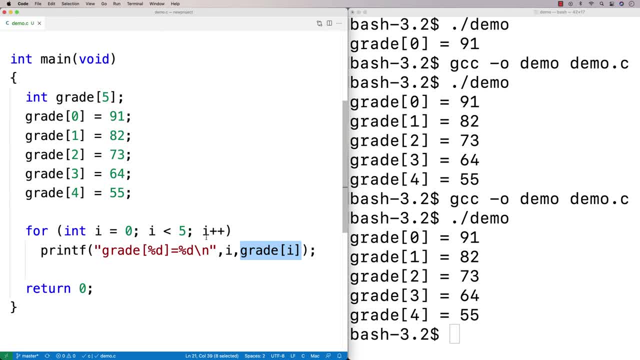 before, But this time it's in a loop where I'm incrementing, i each iteration of the loop from 0 until 5, but not including 5.. So it's going to go up until grade 4.. And if I run this here, 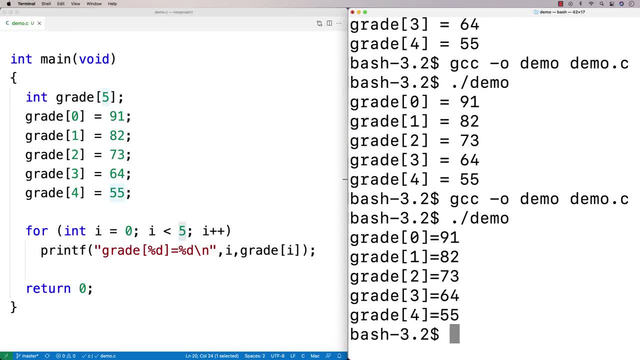 I'm going to get the same output as before. What this approach is. number one: look at how much shorter my code is. Number two: this is going to scale way better Because let's say I add another grade. Let's say that I actually add. 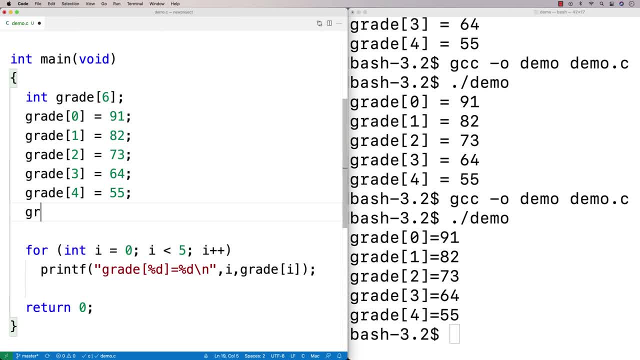 a sixth grade. So I'm going to say here grade 6.. And I'll say grade 6 here And I'll say maybe this one is equal to, we'll say, 43. If I want this code to still work with this new grade array. 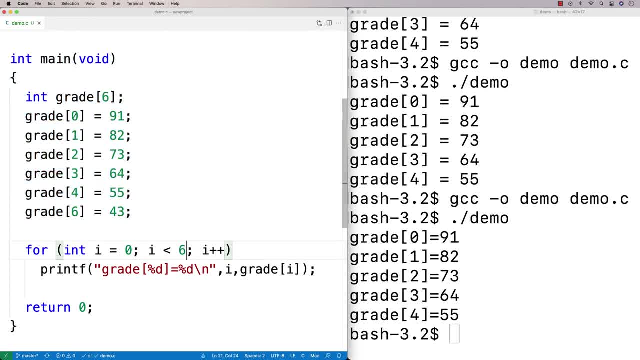 all I have to do is change this. All I have to do is change the sort of length of the array that I'm working with here, And this code is still going to work fine, And it doesn't get any larger, So this is going to scale way better. I could work with larger and larger data sets. 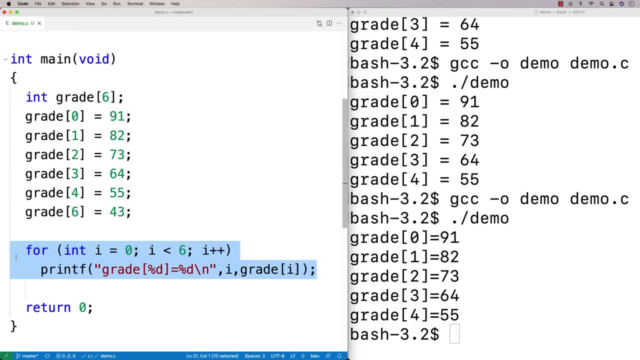 And my code doesn't really need to change much, if at all. And even this here, this number- here I'm kind of hard coding a number in there- We could make that a variable, Or we could use what's called a constant to define that as well, And so we're going to be able to write code to: 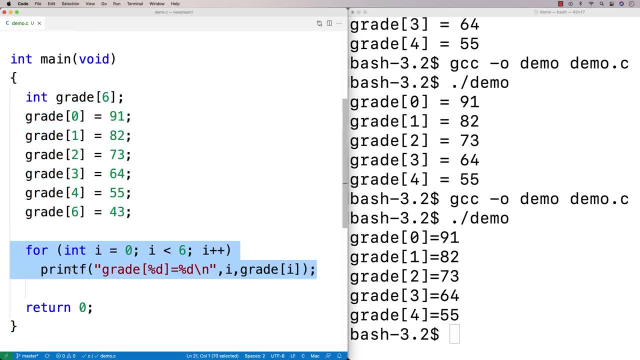 work with groups of data where our code doesn't have to change a lot, if at all, When we make changes to the size of that data. So that's a big thing with arrays And we could run this here just to make sure it's going to work And it says warning here. Oh, you know what? 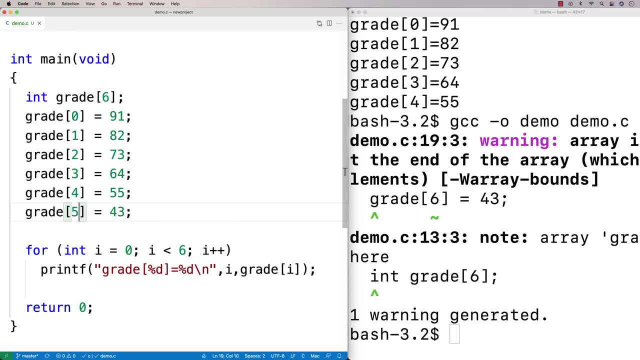 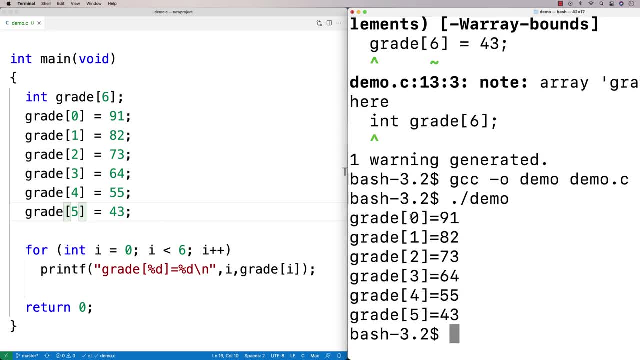 I did. I put grade 6 there. It's grade 5.. It's grade 5, right, Because we start counting from 0.. OK, So I run this here And now we get grade 5 is printed out And it's 43. And that makes. 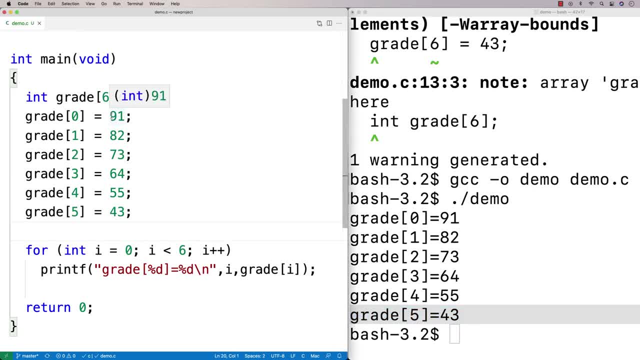 sense And we're happy. Now, what I did here was I declared the array And then I initialized the values in the array individually underneath it. You can do it this way, But there's a couple other ways you could do it that would take up less lines of code. 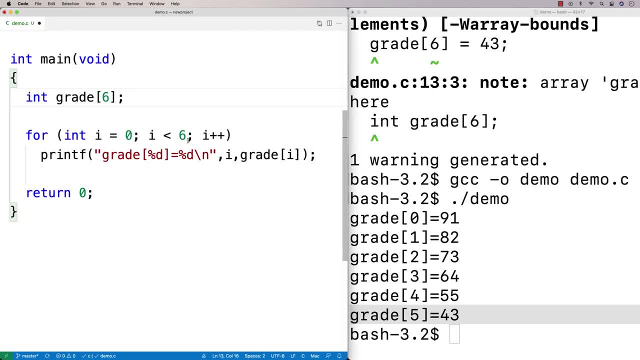 So one way we could do it is this- And I'm going to go back to being a link: 5 array. So I'm going to say here 5 and 5.. We could do it like this. I could say: is equals to squiggly bracket And I 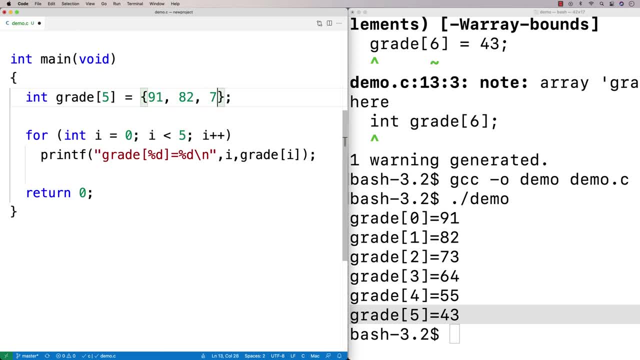 could say here: 91,, 82,, 73,, 64,, 65,, 66,, 67,, 68,, 69,, 70,, 71,, 72,, 72,, 73,, 72,, 73,, 72,, 72,, 73,, 72,, 72,. 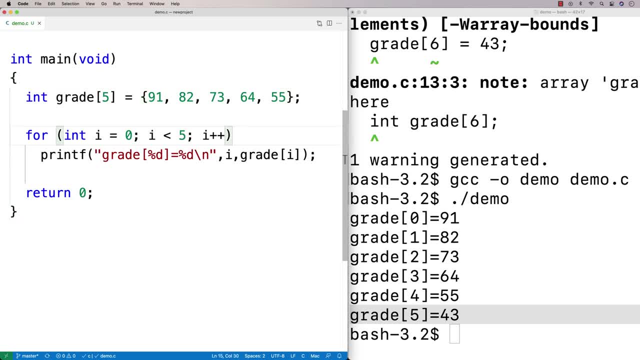 64, 55.. This will actually do the exact same thing. This will actually initialize the grade array with 91 in the first index, 82 in the second index, 73 in the third and 64 in the fourth and 55 in the fifth index, And so we could run this here And we'll get grades from 0 to 4 there. 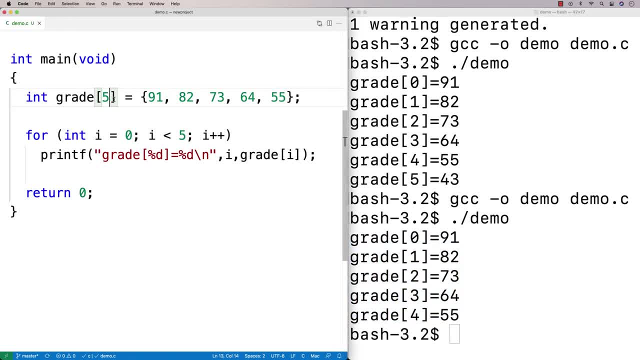 being printed out, And another way we could do it is this: I could actually get rid of this here, I could get rid of the 5 there, And this will also. This will also work fine. This will also initialize the grade array in the same way. 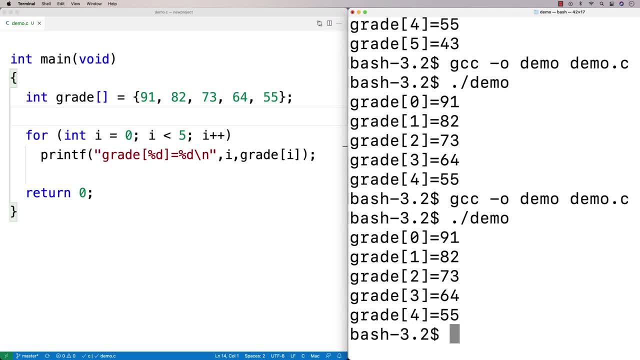 Because basically the C compiler can tell by the number of elements we've got here, by the number of grades we've got here, how big the array is, And it knows that like, okay, they want to make an array of length 5.. So you don't actually need the 5 there. You could actually. 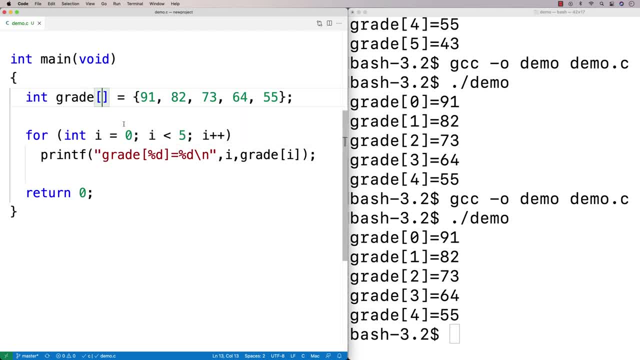 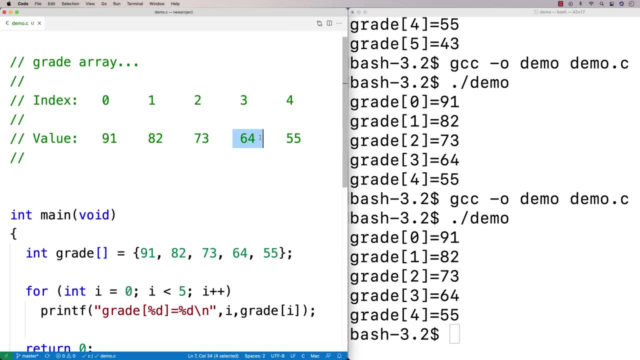 take out that number there and it'll still work fine. So one thing we should discuss is a little bit of the terminology. So the values here. these are typically called array elements. We call these elements of the array because they're the individual things inside of the array. Now another